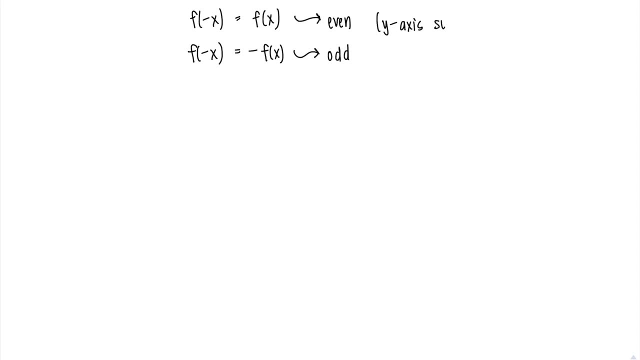 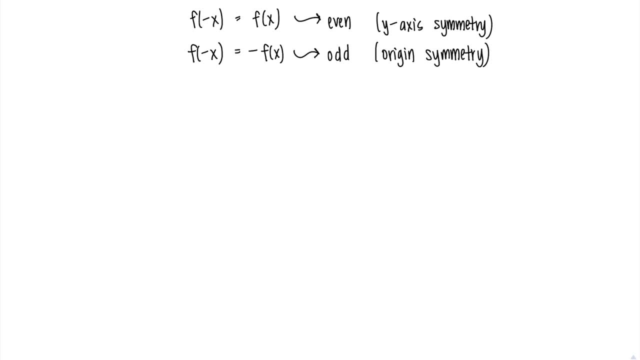 substitute in negative x for x into the function. If it comes out exactly the same as the original f of x, then it was even. And then if it comes out to be the opposite of the original function, f of x, then that means the function's odd. We're going to go through a bunch of examples that are similar. 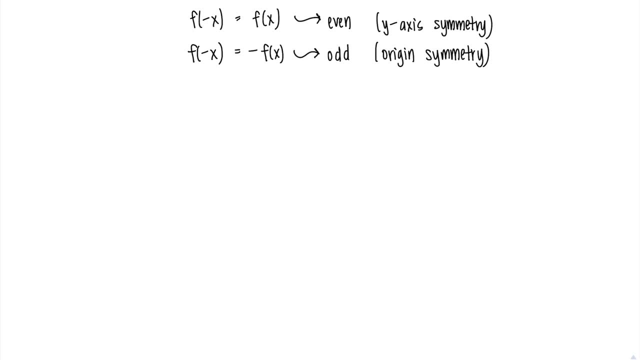 to see the subtleties in what makes a function even odd, or neither. So first example: f of x is equal to 3x squared minus 7.. So we'll substitute in negative x for x, So we have 3. 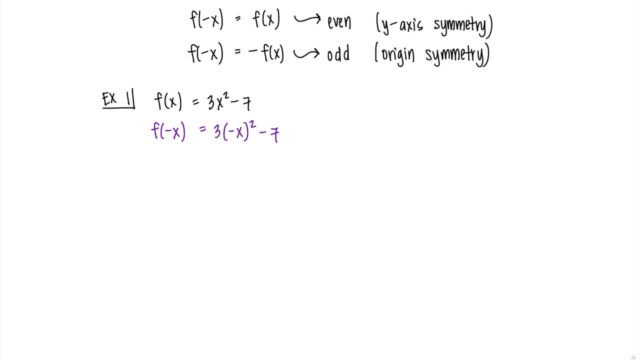 times the quantity negative x squared minus 7.. Make sure you put parentheses around the negative x, because the exponent, the squared term, applies to the negative as well as the x. So if I simplify this now, I'll have 3 times positive x squared. 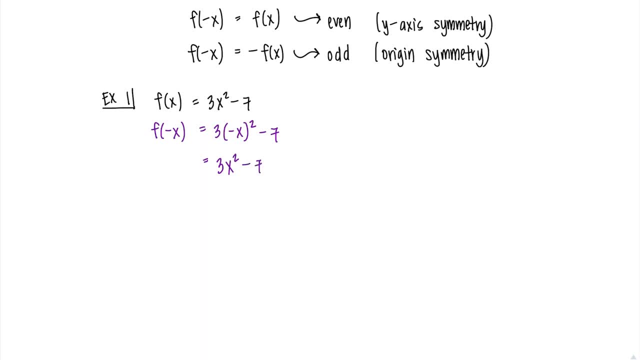 minus 7.. minus 7.. I'm going to compare this result here with my original function and notice it's exactly the same. So this is equal to f of x. That means f of x is even Great. Now what if we change the function just a little bit? 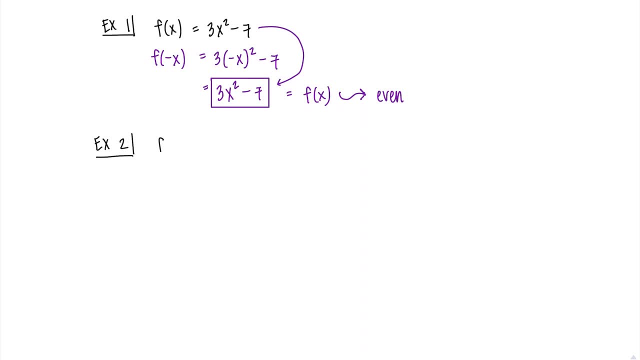 So say f of x is now equal to 3x squared minus 7x. So same test, So substituting in negative x for x, I have 3 times negative x squared minus 7 times negative x. So the negative x squared will become: 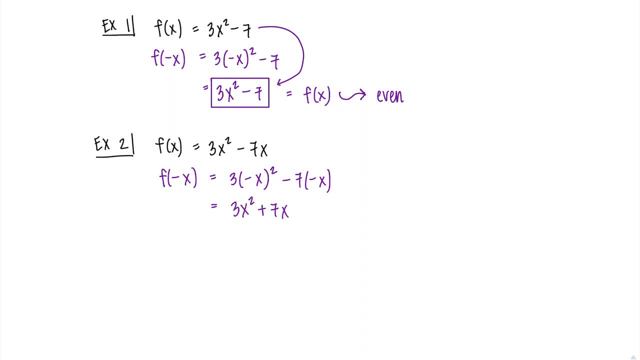 just a positive x squared. So we have 3x squared plus 7x. Now compare this with a positive x squared. So we have 3x squared plus 7x. Now compare this with a positive x squared. our original function f of x, Notice: 3x squared is still positive, but 7x originally was negative. 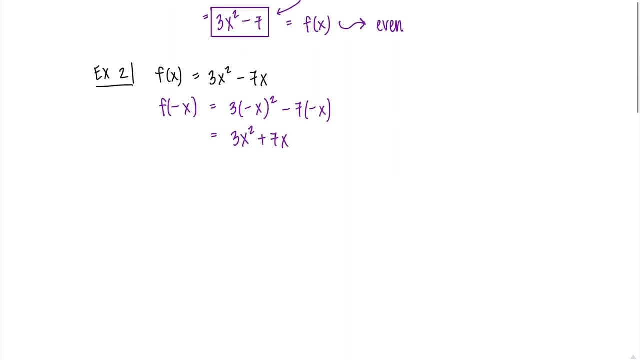 and now it's positive. This is not equal to the same original function. so I know f of x is not even, but maybe you're thinking it's odd. Well, if it was odd, negative or the opposite of f of x would mean that I would take the entire function and multiply by a negative and that would result in negative 3x. 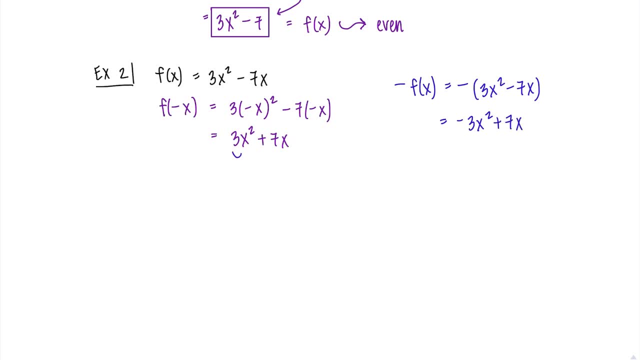 squared plus 7x, which is not what we see here. So that means this function is neither. Alright, a couple more examples. Let's look at some rational functions. First one, we'll call it g of x. g of x is equal to x cubed over x squared. 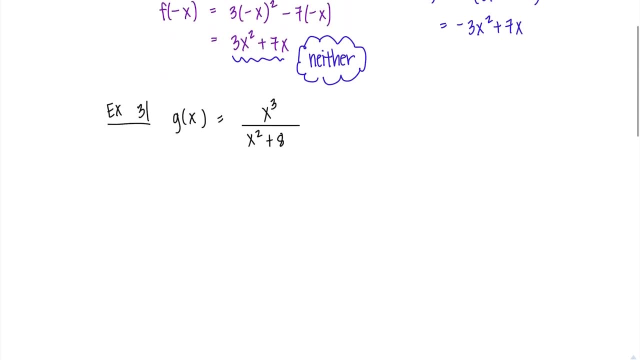 Plus 8.. Okay, so, starting off same as the other examples, I'm going to substitute in negative x for x, So g of negative x is going to be negative x cubed over, negative x squared plus 8.. And then in the numerator I'm still going to have a negative sign left over, since it's being raised. 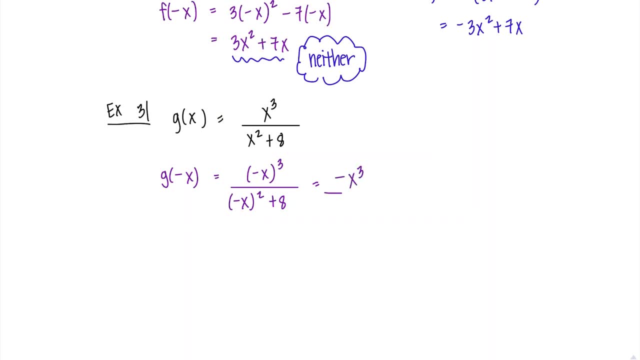 to an odd power. So that's negative x cubed, And then the denominator will have positive x squared plus 8.. Okay, now let's compare this with our original function. The denominator looks exactly the same. There's an extra negative in the numerator, But remember this negative. we can. 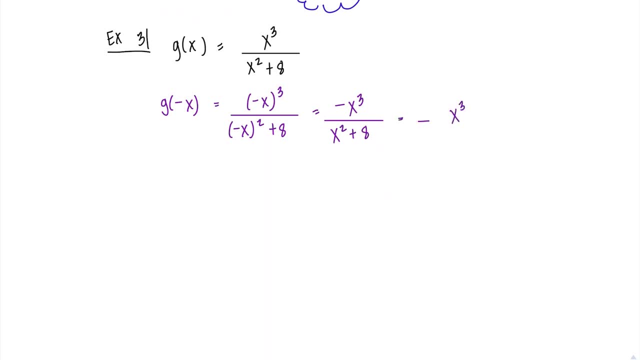 rewrite it outside the entire expression and it would still be equivalent. And if you notice, this is the original function: g of x. So we've just shown that g of negative x is equal to negative g of x. By definition, this means our function is odd, So keep in mind, you can move. 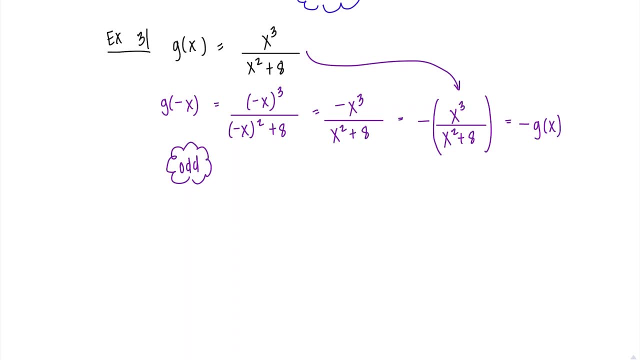 that negative when necessary. That negative in the numerator applies to the entire expression. Good, Now what if the function looked a little different? What if there already was an extra negative in the numerator? So what if we had g of negative x is negative, x cubed over x squared plus 8? Would that affect whether the function is even odd? 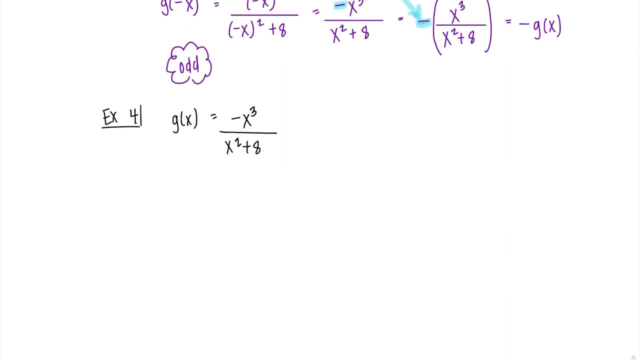 or neither. Take your guess. and then let's check algebraically now. So we have g of negative x equals negative, negative x cubed over negative x squared plus 8.. Now I'm going to have a positive x cubed in the numerator. 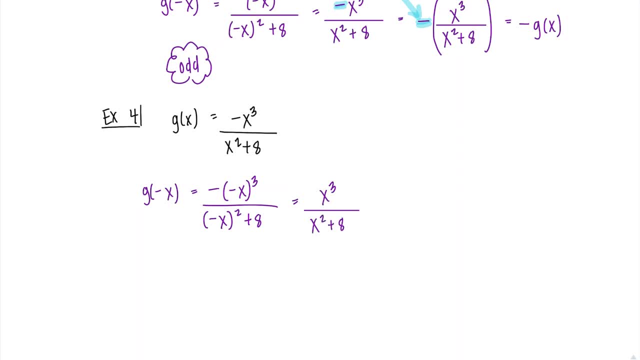 squared plus 8.. Now compare this result with our original function. The denominator looks exactly the same, but now the negative is gone in the numerator. But isn't this exactly equal to the opposite of our original g of x? This was my original g of x, and now I'm left with the opposite of it. That means 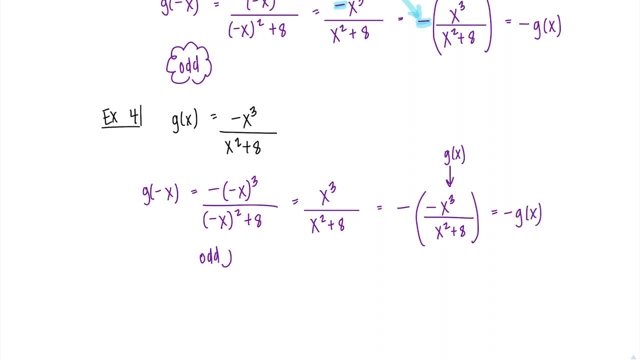 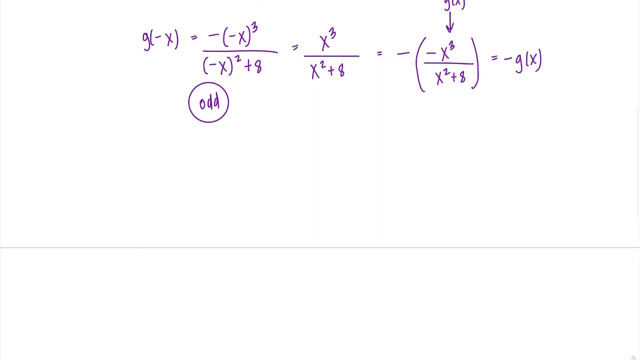 g of x is still odd. Okay, so that can be a little tricky for some students to see, so just make sure you remember the definition and apply them strictly. Okay, continuing on, let's look at some radical functions. Example 5, say f of x is equal. 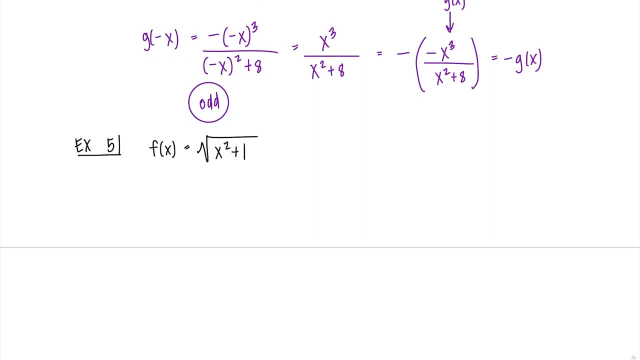 to the square root of x squared plus 1.. So same start: f of negative x is going to equal the square root of negative x squared plus 1.. And then, if I simplify underneath the radical now, I'm going to have positive x squared plus 1, and this is exactly the same as what we started. 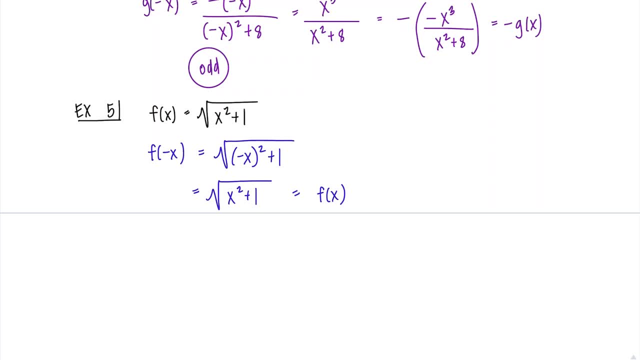 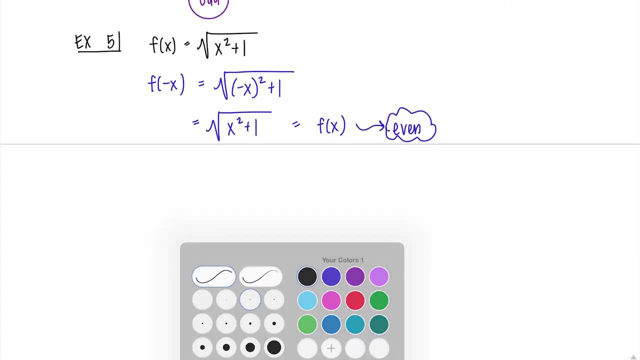 with our original f of x, So that means our function is even Beautiful. Okay, let's change up f of x just a little bit, and then we're going to get our wee bit and see what happens. So now f of x is equal to the square root of x, cubed plus 1.. 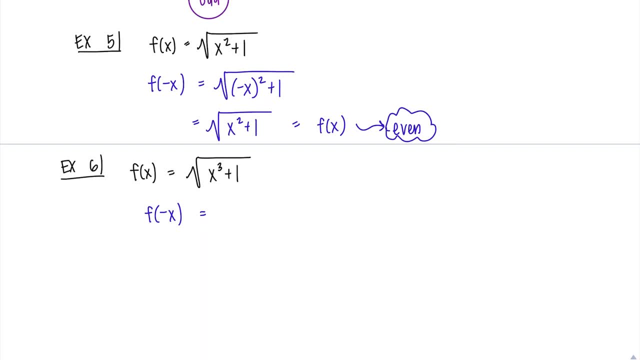 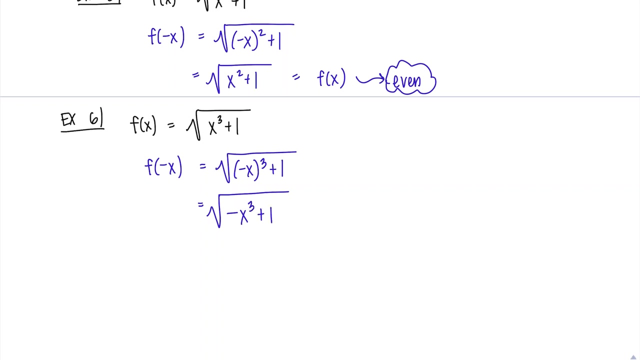 All right, that means f of negative x is going to equal the square root of negative x cubed plus 1.. Now, this time the negative will stay underneath the radical. I have negative x cubed plus 1.. Now, this is clearly not the same as the original f of x that we started with. So we know our. 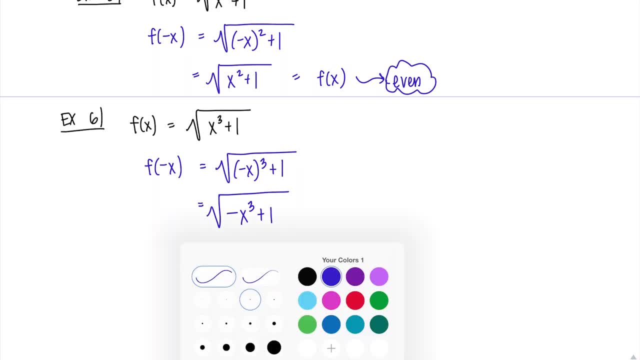 function's not even. But maybe you're wondering if it's odd. Well, if it was odd, we would be left with negative f of x, which would be negative square root of x cubed plus 1.. But that's clearly not what we have here. We have a negative underneath the radical next to or being applied. 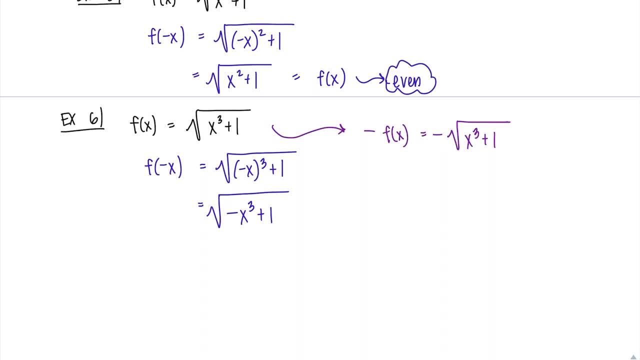 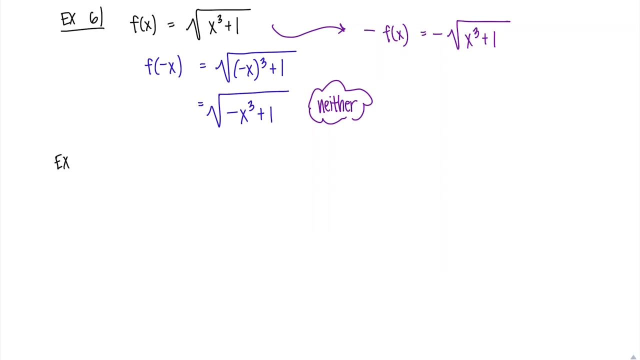 to just x, cubed, not outside, Or applied to the whole radical. So in this case, our function is neither, Neither, neither, whatever you like. Okay, what if we had a different index on our radical? So what if f of x was equal to the cube? 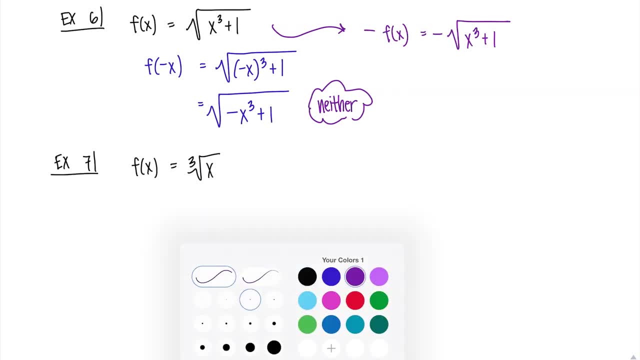 root of x. Well, in this case, f of negative x would equal the cube root of x, cubed plus 1.. And since the index is odd, that negative can come outside. If you need to remind yourself why, remember I can rewrite this as negative 1 times x. And since our index is odd, we 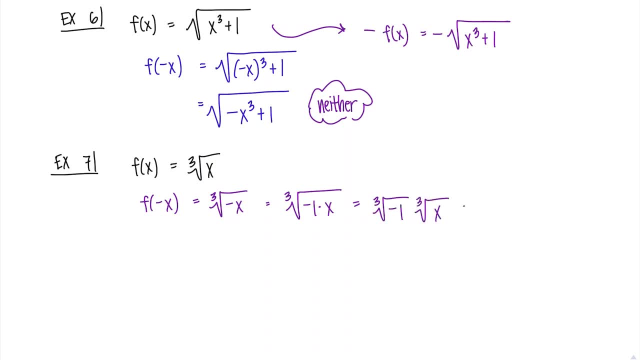 have the cube root of negative 1 times the cube root of x. So this is negative cube root of x. Now compare this result with our original function, f of x. right here. Well, there's f of x and I have an extra negative outside. This is equal to the opposite of f of x, Which means this function is: 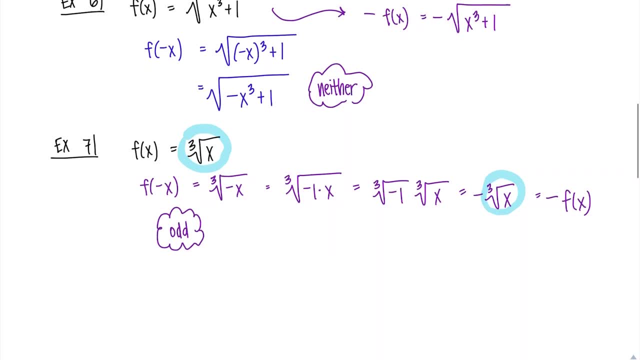 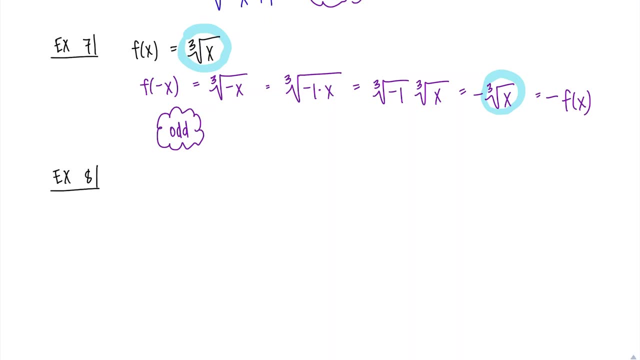 odd. For the grand finale, let's look at an absolute value function. So we'll have: g of x equals 5x over the absolute value of x. Alright, Alright. So g of Negative x is going to equal 5 times negative x over the absolute value of negative x. 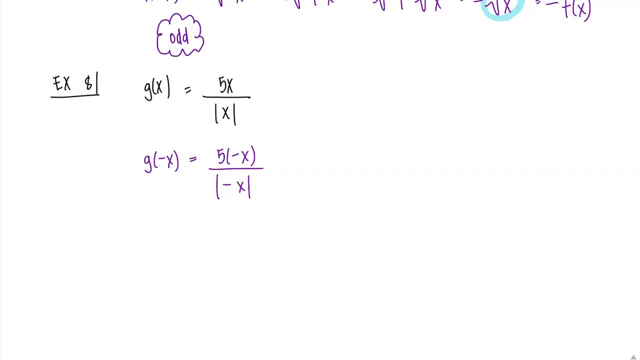 Now the numerator is pretty straightforward in simplifying. It's just going to be negative 5x, But the denominator: remember, when you have absolute value of negative x, the negative will go away, but the absolute value still needs to be there.